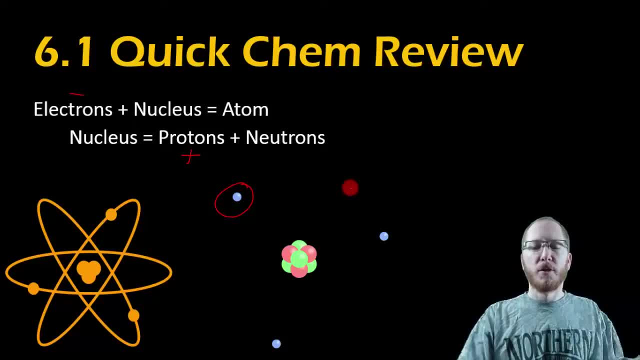 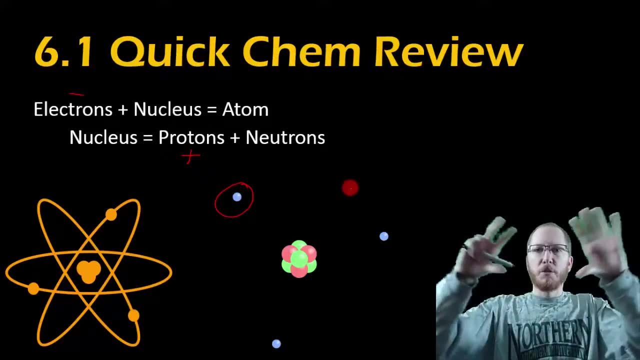 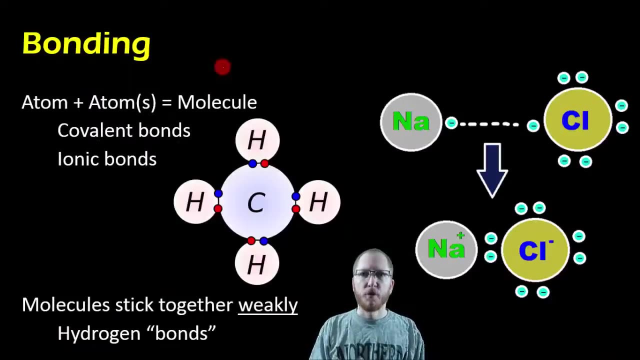 The neutrons will actually play kind of a key role there. So this is the basic structure of an atom: Protons and neutrons in the nucleus, tiny dense part in the center. Then you've got a large part outside of that. that's primarily empty space with some electrons flitting around in there. So now we're on to chemical bonding. So chemical bonding is when we take multiple atoms and we stick them together using these things called bonds to form molecules. Right? So this is just going to be multiple atoms together. Now, when we want to stick two atoms together, 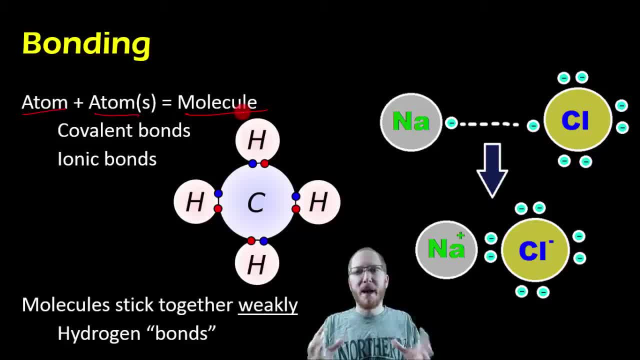 there's two basic ways we can bond them that we'll ever really see in biology. That's covalent bonding and ionic bonding. Now I will tell you, covalent bonding is by far, hugely by far- the most common one that we're going to see biologically. So this is going to be our main emphasis, And the way this works is you have atoms that want to have a specific number of electrons in their outer energy shell to feel stable, And that number is usually eight. Now there's one exception: 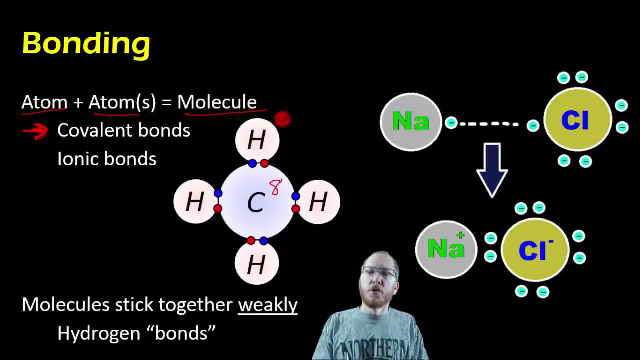 That's going to be hydrogen, who only wants two. So carbon wants eight electrons, but it only has four. So let's just look at these red ones and say: the red ones are carbon's original four valence electrons. So it needs four more to be stable. So what it tends to do is form four covalent bonds where it will share one of its electrons with somebody else who also shares an electron. And so in this case we've got hydrogen that has one electron. he wants two. So by sharing this electron, by kind of putting it into the 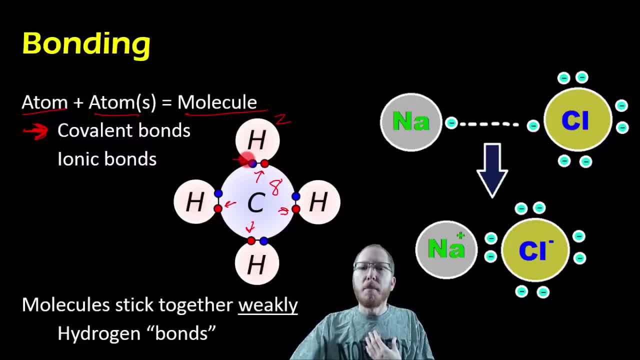 pool. carbon also shares one electron. So they both look at this region where they're expecting to see their electrons. and they both see two electrons, So they're both happy. Hydrogen wanted two. it has two. Carbon, by forming four of these bonds, looks around and sees two, two, two, two, four sets of two. It sees eight electrons. So it says, hey, I'm stable, It doesn't matter that they're being shared as far as it's concerned. Within its electron cloud it sees eight outer electrons. 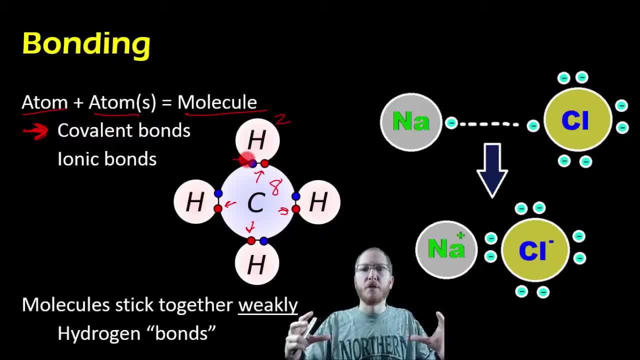 So it's content, just like hydrogen within its electron cloud sees two electrons, which is what it wants, So it's content. These are strong bonds. This allows these chemicals to be much more energetically stable, which is a lower energy level. So that makes them- what some people say is happier. They don't have emotions, But really what they're saying is it makes them more stable. Now, with ionic bonds, what happens is you've got somebody that's so far away from getting an octet, which is the stable arrangement, that their fastest way to get to an octet is. 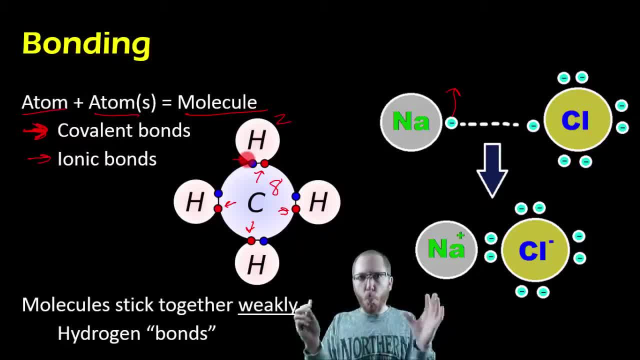 actually to ditch the electron that they have, this one outer electron, because underneath that one outer electron is a whole other shell that's full, which is stable. So instead of trying to collect extras to get a full set, they're just like I can get a full set if I just get rid of one or two electrons. So in the case of sodium Na, this guy has one valence electron which is just not stable, so it just ditches it. It just wants to find somebody to donate it to. just saying, take it. And so it donates this electron to somebody who's almost stable. 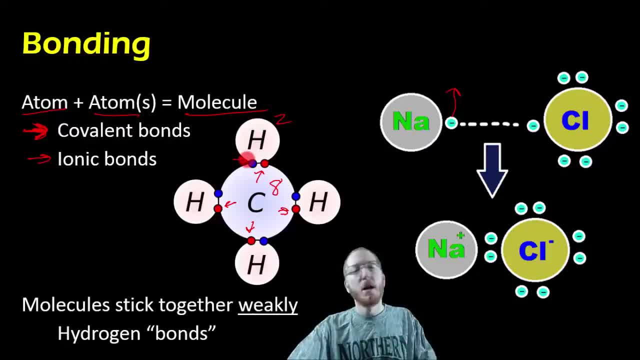 It's almost got a full set. In this case we have chlorine that we're using, but it could be something else- iodide oxygen. There's lots of guys that have six or seven valence especially that really want those, And so by giving it that electron, chlorine's now stable. Sodium is now stable. They're just ions. So we now have a sodium ion, which is one positive because it lost a negatively charged electron, And we have what we call a chloride ion, which is basically going to be one negative because it gained an electron. 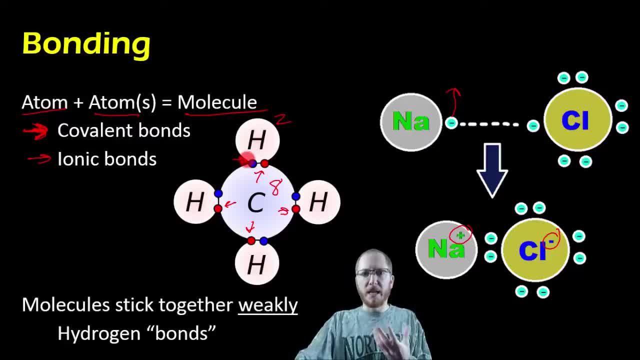 So then you might be like: well, why are they attracted? then They just donated it. That doesn't mean that you're connected. Well, the charge is what causes this, If you remember that opposite charges attract. So now we've got this positively charged guy that's near this negatively charged guy, so they're going to attract each other. Now it doesn't have to be this exact sodium You know you could have, where there's a bunch of sodiums and they kind of shift around a little bit. originally It's not like they have to exactly bind to the guy they donated it to. But you are going to see that these positive charges are going to attract each other. 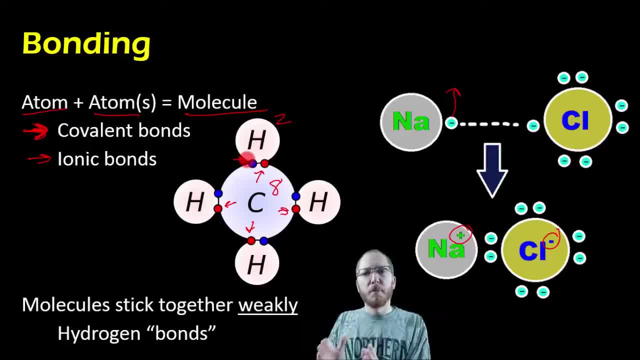 So these positively charged- we call them cations- are ultimately going to be attracted to these negatively charged anions, And it's going to be a strong attraction. I mean, this is going to be something where they're held together tightly. Now, for biological purposes, though, because you have a positively charged and negatively charged ion, and because water, a substance that we're made up of a lot of, happens to be partially charged, if you put ionic substances into water, they tend to dissociate. That means they break apart. 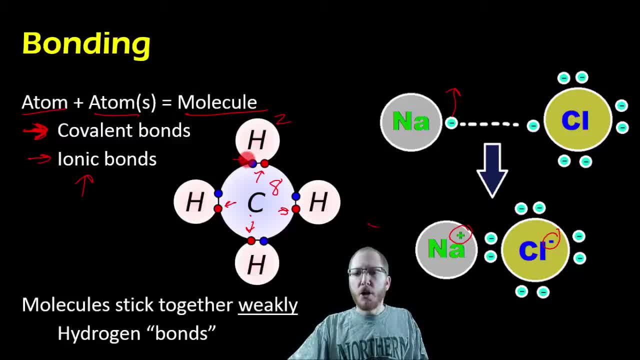 And these ions just start to. instead of interacting with each other, you'll see that these ions start to interact with water instead. And so if you put salt in water, you'll see the salt will dissociate. It'll kind of seem to break apart in the water. 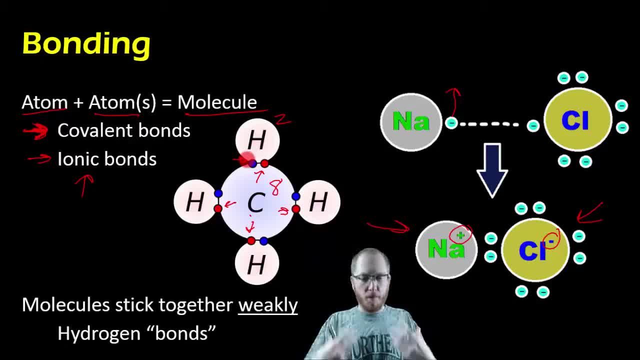 So this is why we don't talk about ionic bonds as much for biological purposes, Because in most cases when you put ions into our bodies they tend to just dissociate and kind of spread apart into our body fluids, You know, like blood etc. 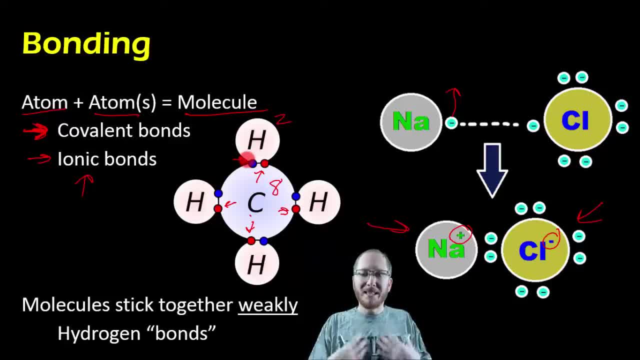 So this can be important because we can see that these ions just start to interact with each other. We can still move those ions around our body, It can still matter, But they're not normally going to be like in crystallized ionic form inside of our body. 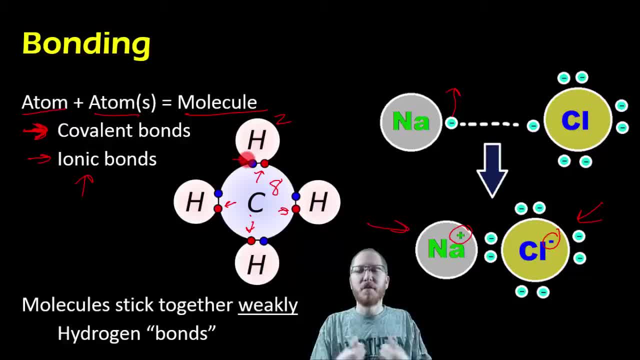 There are some cases when they do things like gout, where you get these crystals that form that are not fun, But that is typically more of a rarity and it's more of a problem when it happens than the de facto of what we expect. 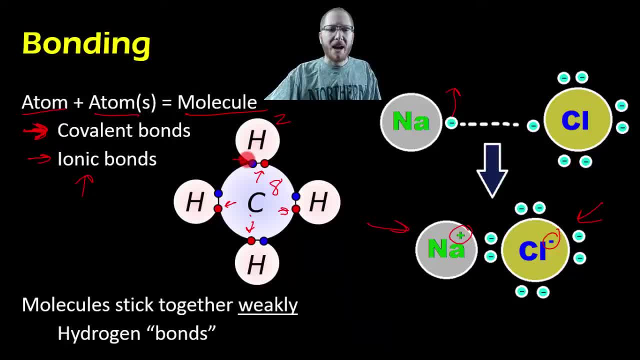 Now we do have in some cases where we have actual separate molecules that stick together. So this would be like if I've got a series of waters that we're going to talk about in 6.3. But if I have a series of these separate water molecules, each of these is its own separate thing that's covalently bound to each other. 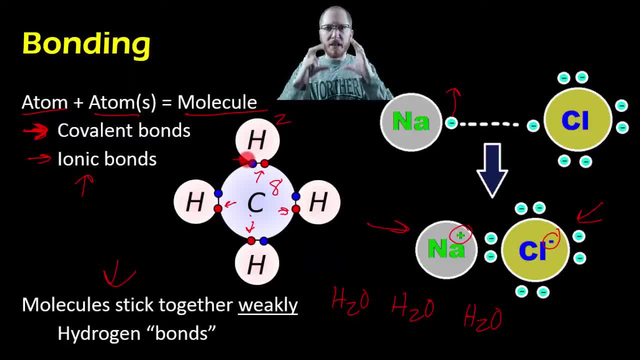 So two H's are bound to an O. that's one unit, that's one molecule. But sometimes we'll get where these molecules can weakly attract each other. So that means this: one H2O can weakly attract another H2O. 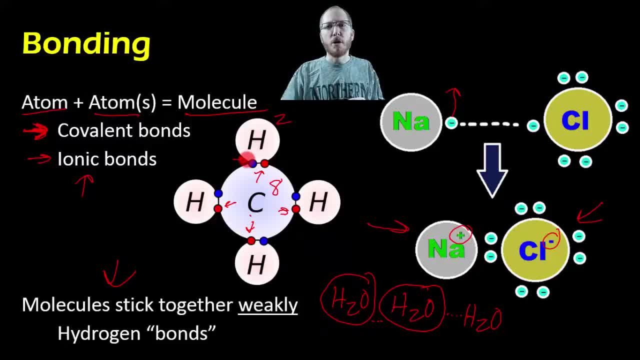 And so sometimes they'll show that with like dotted lines to show it's kind of weaker. These are not as strong as chemical bonds, nowhere near as strong. But you can get these attractive forms, You can get these attractive forces that help stick together separate molecules. 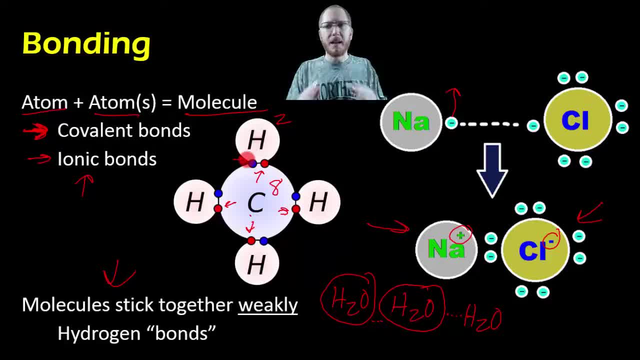 The most common and the strongest of these will be the hydrogen bond, which is misnamed. It's not a bond. It happens to be the strongest attractive force between molecules, But it's still only probably about 5% as strong as a covalent or an ionic bond. 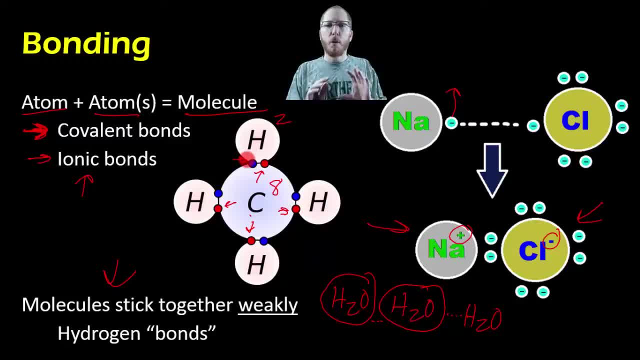 So much, much, much, much weaker. There's other forces that exist that we won't get into. that also kind of help these things stick together. But keep in mind that even separate molecules can actually help stick together. It's just not going to be as strong. 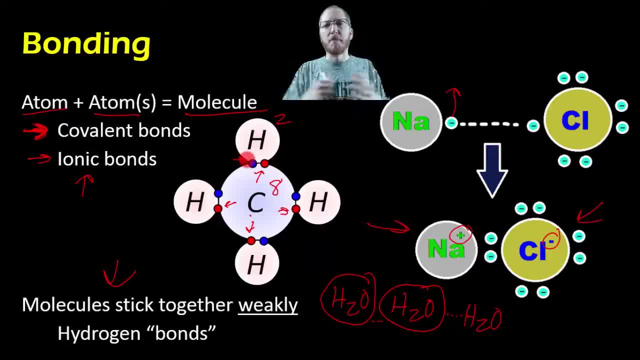 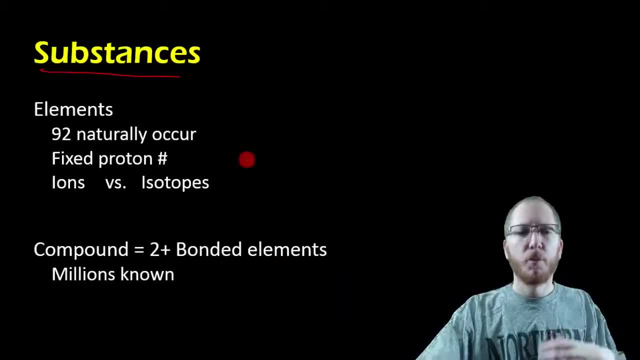 It's much easier to separate those guys versus a covalent or ionically bonded substances, which are very difficult to break in most cases. Now, lastly, we've got this idea of substances, So oftentimes you'll see this referred to as pure substances. 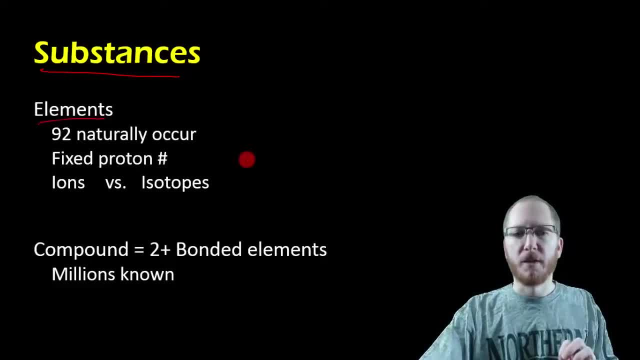 So on Earth we can find the simplest pure substances are elements. So we can have oxygen, which is oxygen. You know, that's just what it is. It's the smallest we can break something down and still keep its properties. So we call those elements. 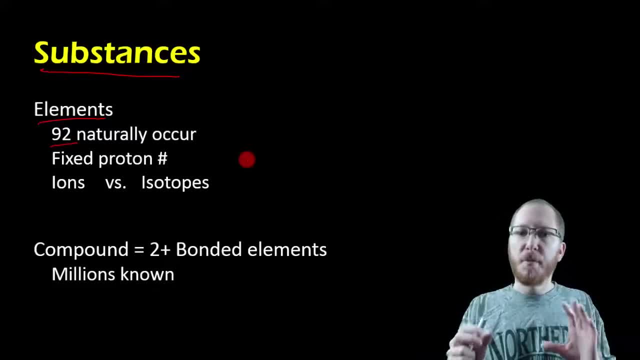 And there's 92. We find in nature. There's others that are man-made But for biological purposes. we normally don't deal with those as much because they're not in nature And the idea of what makes an element an element is they have a specific number of protons. 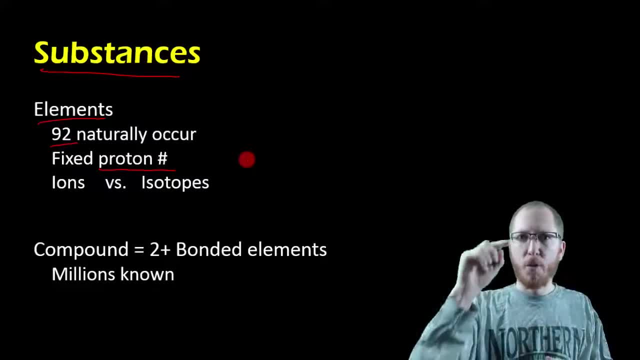 So if you look on the periodic table, there will be an atomic number that it's ordered by 1, 2, 3, 4, 5, 6, 7, 8, blah, blah, blah. That's the number of protons that it possesses. 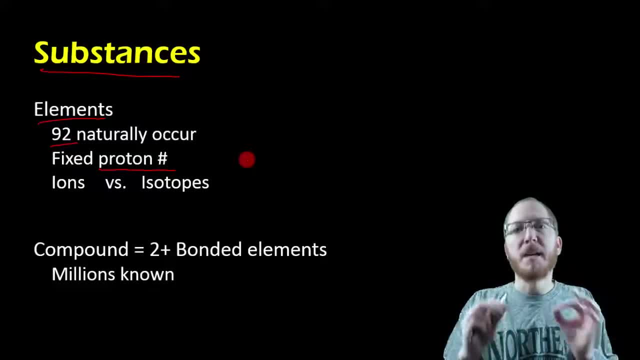 If I were to remove a proton from an atom, from an element, it would become a different element. So for identity purposes, just keep in mind, protons are what matters, because we can add or remove electrons And that's what gives us ions. 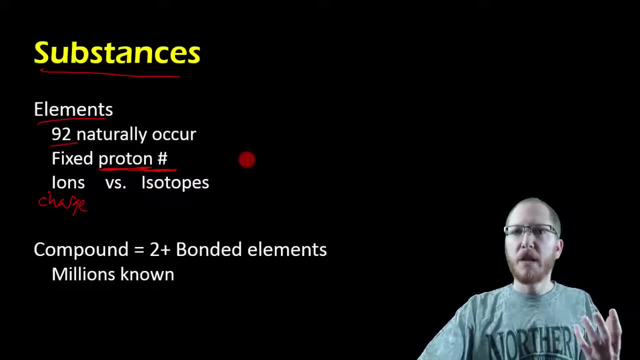 That's what ultimately gives something charge right. I didn't change the protons. There still might be 10 protons, But if I take away 2 electrons you're now 2 positive And the reason for that is because you have 10 positive charges- protons- and 8 negative charges- electrons. 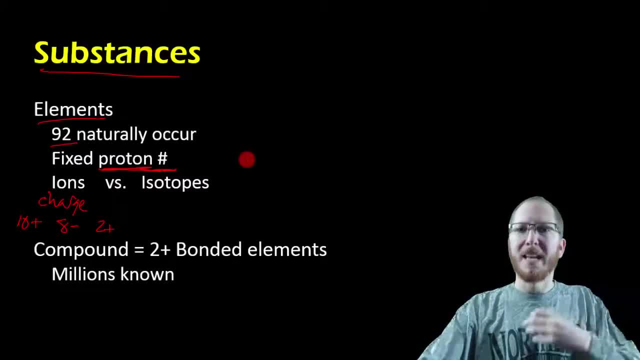 So if I just do the basic math, I'm 2 positive, So we can add electrons, remove them and give something charge. We'll also have isotopes that we deal with in later sections, And this is basically where you have the same number of protons, the same number of electrons.